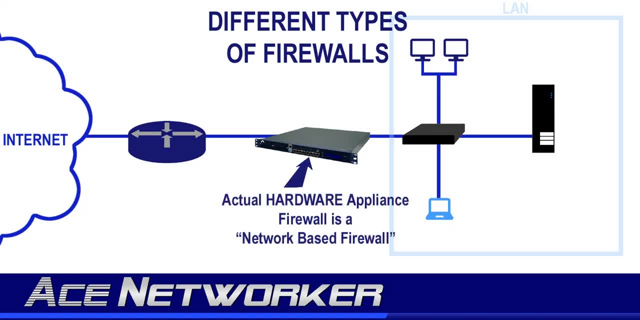 or appliance firewall, a device that is built as a firewall, in other words, that's why it was built. it is known as a network-based firewall. Typically, you will see a network-based firewall placed between your internal LAN and the external network. Again, 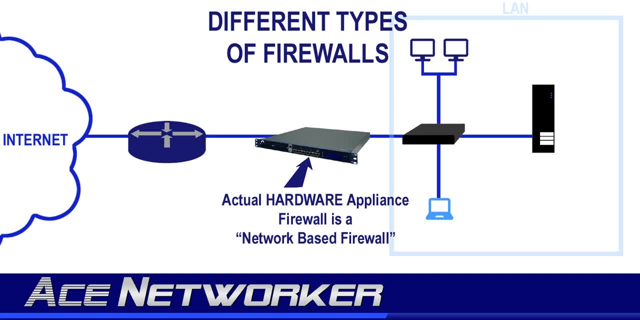 usually the internet. If you use or operate a network-based hardware firewall, it is usually used as the first line of defense on your internal network. Network-based firewalls really tend to serve this purpose well enough to allow for a network-based firewall to be used for any type of 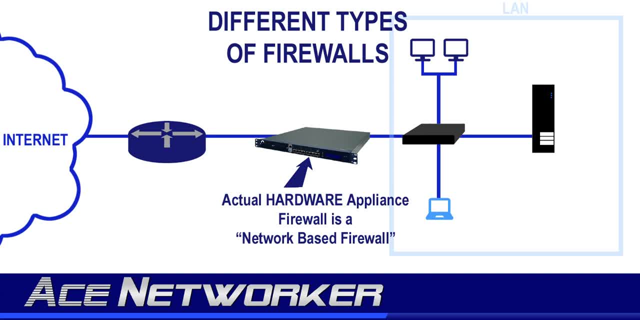 attack. However, they are of little use to any attacks coming from inside your local area network. This is where host-based or software firewalls are used. Host-based software firewalls are installed on a host to provide firewall services for just that machine. A good example. 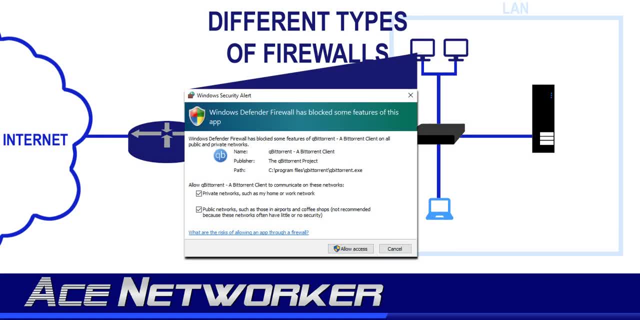 of a host-based software firewall is the Windows firewall found and used on Windows operating systems. A good example of a host-based software firewall is the Windows firewall found and used on Windows operating systems. The most often encountered firewall a network admin or technician will deal with is the host-based software firewall. You will also see firewalls that are known as. 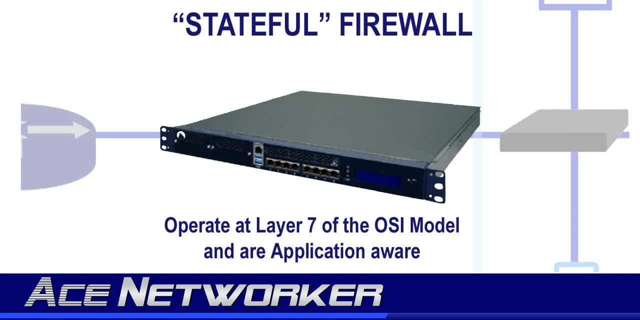 stateful firewalls. Stateful firewalls operate at layer 7 of the OSI model and they are application or context aware. A stateful firewall uses what's known as deep packet inspection, DPI, to filter the traffic based on the service or the application where the traffic originated. A good example of 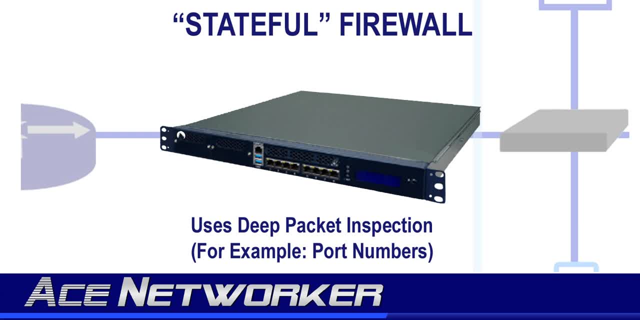 where deep packet inspection comes in handy is on something like bit torrent that used to be used that could overload your network because it used port hopping. A stateful firewall using deep packet inspection is invaluable in that type of scenario. And last but certainly not least, you will see what. 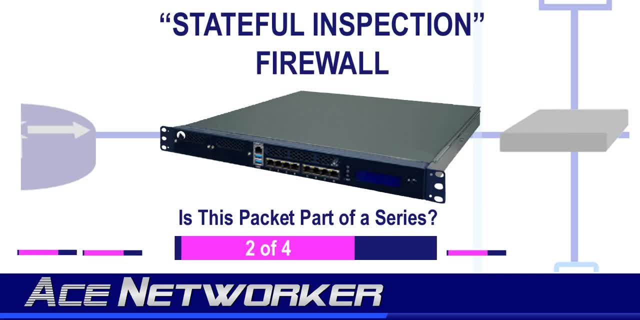 are called stateful inspection firewalls. This is typically on the newer, latest firewalls that you see out there. A stateful inspection firewall is capable of being able to tell if a packet is part of an existing connection. In other words, firewall can look at a packet and know what that packet state is in relation to other packets. Now 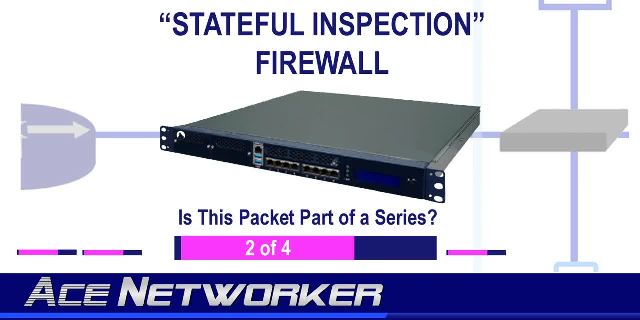 I'll get into more detail on things like windowing used on session management across a connection when it comes to session layer and the transport layer in the OSI model. but for now just know that a stateful inspection firewall can tell and be aware of these multiple packets in a connection.